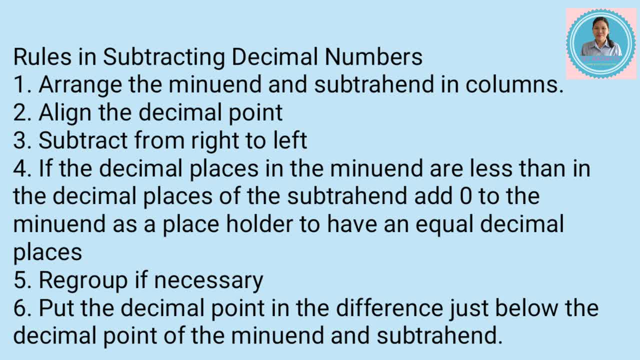 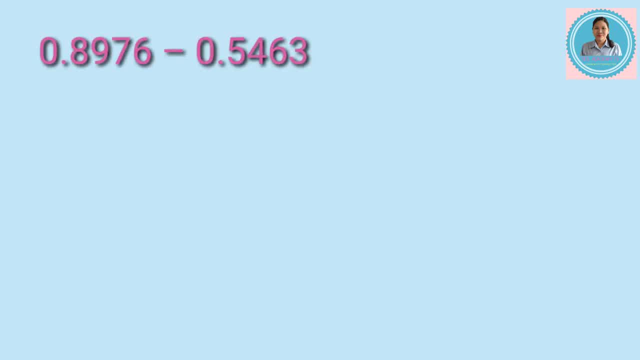 Six. put the decimal point in the difference just below the decimal point of the minuend and subtrahend. Okay, Let's arrange the numbers in columns. The minuend is EIGHT THOUSAND NINE HUNDRED SEVENTY-SIX, TEN THOUSANDTHS, and the subtrahend: 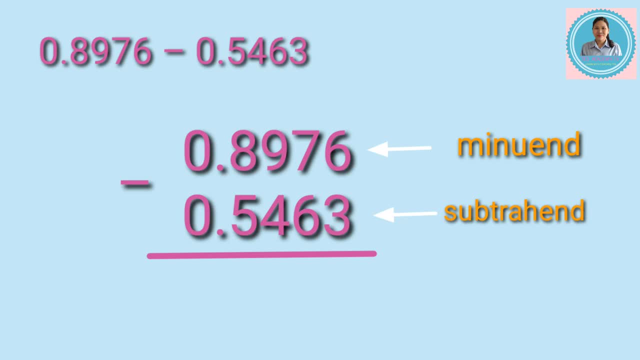 is FIVE THOUSAND FOUR HUNDRED SIXTY-THREE TEN THOUSANDTHS. Okay, Let's arrange the numbers in columns. Number five regroup if necessary. We have DECREASED three, eight hundred thousandths. 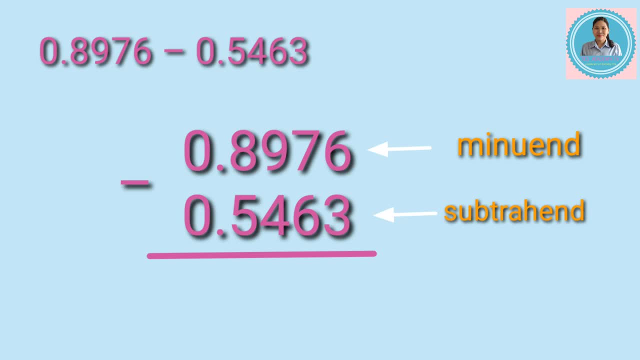 Let's subtract now. We will begin subtracting from right to left Subtract and completely MBAT for five elements. 8 minus 5 equals 3.. Since there is no numbers in the whole number to be subtracted, so we will just copy 0.. 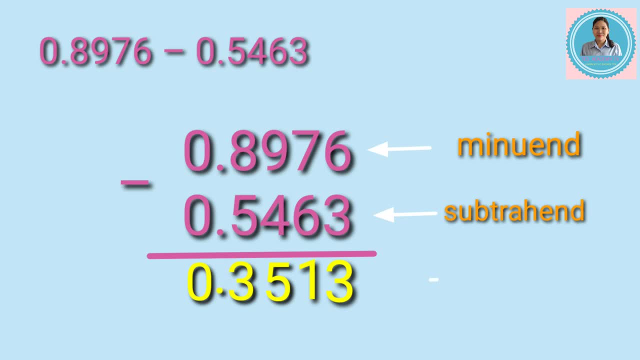 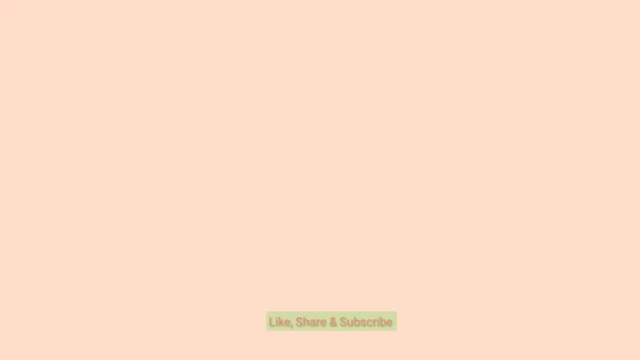 And then put the decimal point in the difference just below the decimal point of the minuend and the subtrahend. So the difference is 3,513 ten-thousandths. Let's have another example: 9,123 ten-thousandths minus 5,876 ten-thousandths. 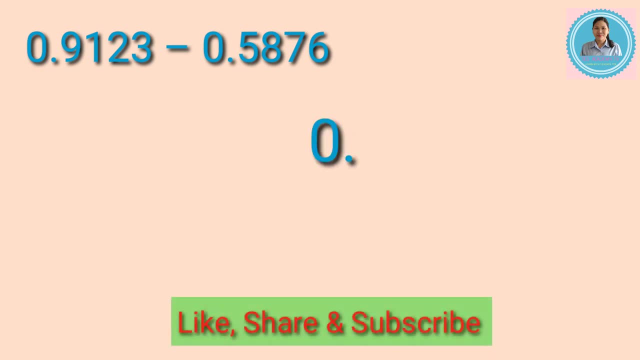 Okay, First let's arrange the minuend and the subtrahend in columns. This is the proper arrangement of the numbers. Now let's subtract from right to left. So let's subtract: 3 minus 6 cannot be because 6 is greater than 3.. 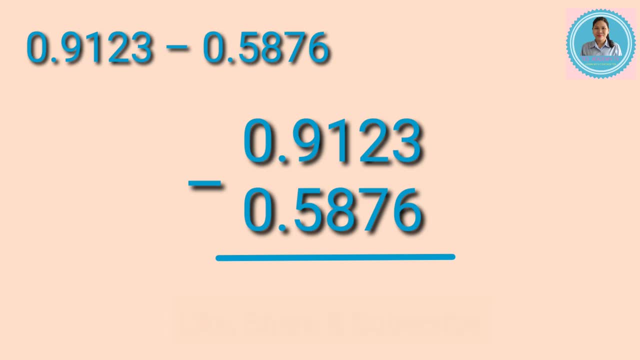 So in this example we need to regroup. We will borrow from the next digit to the left. So we will borrow from 2.. 2 will become 1 and 3 becomes 13, because the number that we borrowed is 10.. 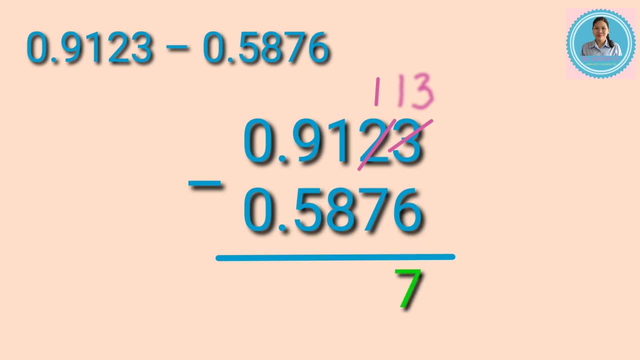 Okay, Subtract now: 13 minus 6 equals 7.. Subtract 1 minus 7 cannot be, So. we need to borrow again from the digit to the left, which is 1.. So 1 will become 0.. 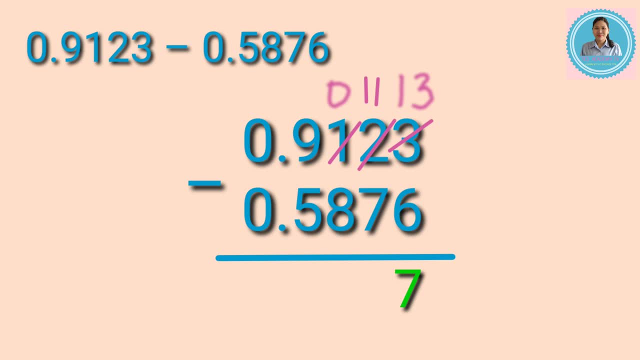 And the number 1 that we borrowed becomes 11.. So 11 minus 7 equals 4.. Next, 0 minus 8 cannot be, So we need to borrow from 9.. Okay, So let's borrow from 9.. 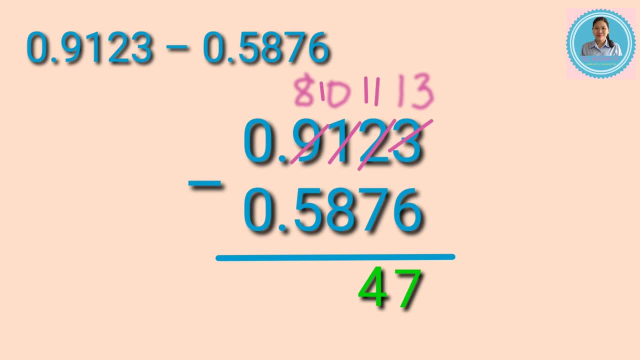 Okay, 9 will become 8 and 0 becomes 10.. 10 minus 8 equals 2.. And then subtract: 8 minus 5 equals 3.. Since there is no whole number to be subtracted, then let's write 0.. 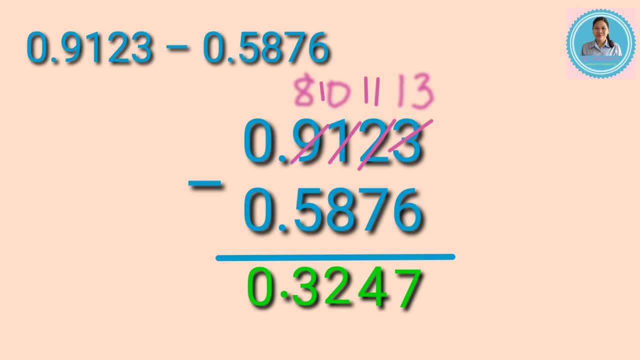 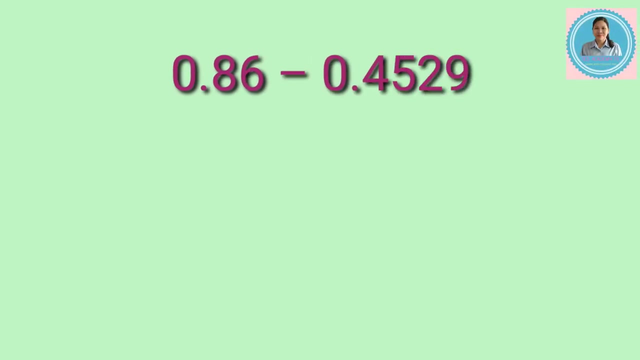 And then put the decimal point in the difference. So the answer is 3242.. So the answer is 3247 ten-thousandths. Another example: 86 hundredths minus 4529 ten-thousandths. Okay, 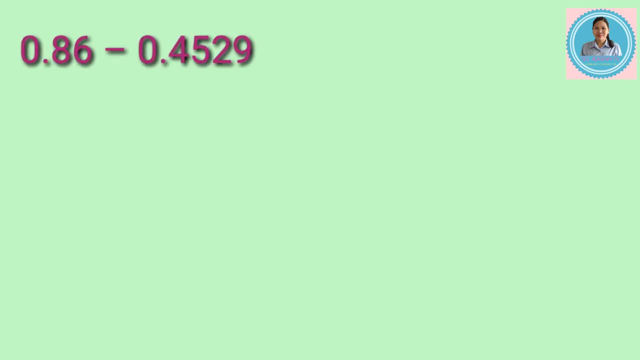 First step: Let's arrange the minuend and the subtrahend in columns. Let's align the decimal point and the digits according to their place value. Okay, This is the proper arrangement. This is the proper arrangement of the numbers. 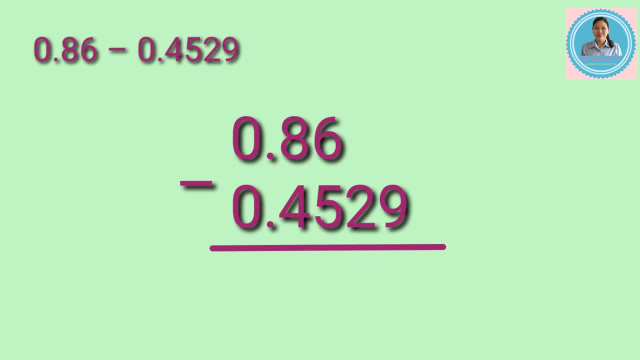 As you can see, there are only two decimal places in the minuend And there are four decimal places in the subtrahend. Okay, In this example we need to add zeros as placeholder to make the decimal places of the minuend and the subtrahend equal before we can subtract. 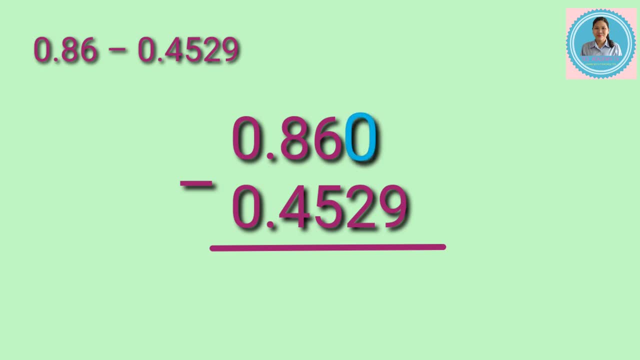 So let's add two zeros in the minuend. Okay, Now the minuend and the subtrahend have unequal decimal places, So we can subtract. now Let's subtract from right to left. Okay, Zero minus nine cannot be. 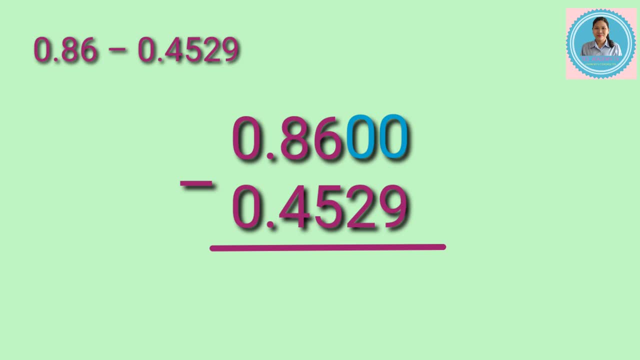 So we need to regroup. Let's borrow from the next digit to the left. But since the next digit is zero, so we need to proceed to the other digit, which is six. So we will borrow from six. Six will become five, the zero in the thousandths place will become nine and the zero in the ten thousandths place becomes ten.